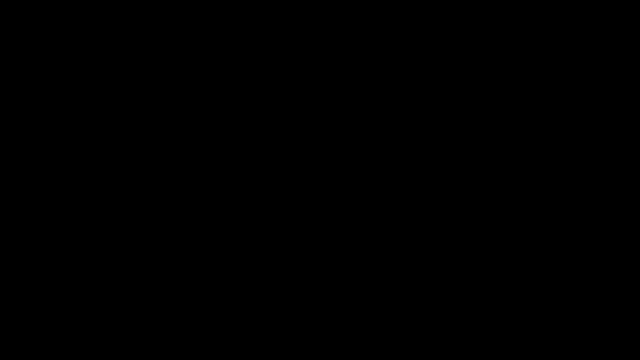 In this video I want to review some basic information, That is, the difference between an altitude, a median, a midpoint, a perpendicular bisector and an angle bisector. So consider the triangle ABC And let's say that BD is a median. 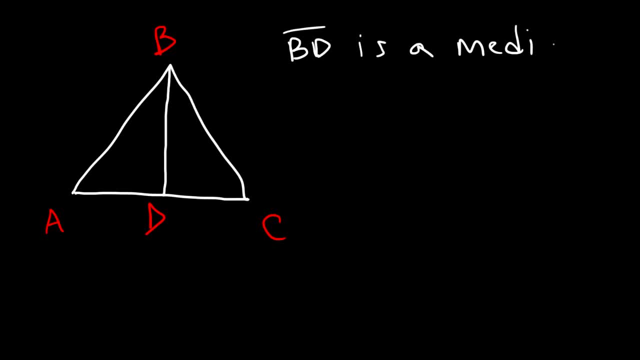 So if BD is a median, what conclusions can we draw? Well, we need to know what a median is. A median is a line segment that extends from the vertex of one side of the triangle, so vertex B, to the midpoint of the other side. 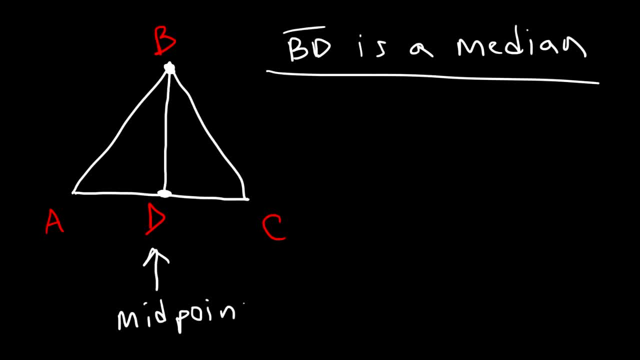 So D is the midpoint of segment AC. A midpoint is basically a point in the middle. The midpoint breaks the segment into two congruent segments, which means that AD is congruent to AC, And that's all you need to know about a median. 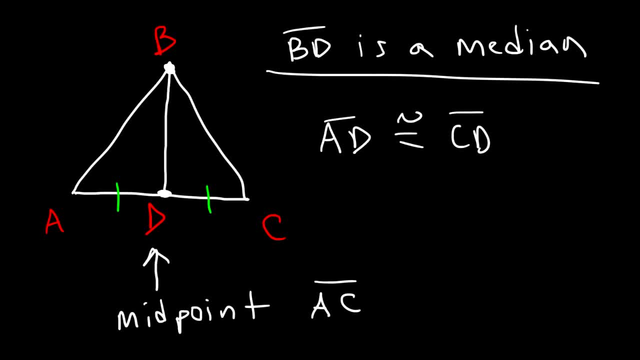 A median is simply a line segment that connects the vertex of one side of the triangle to the midpoint of the other, And the median will bisect that segment. So you can think of the median as a segment bisector. It splits the segment into two congruent parts. 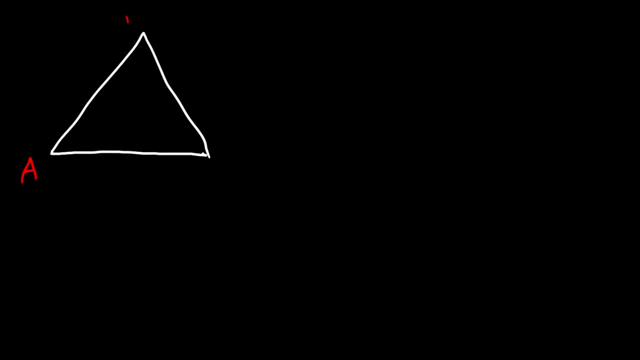 Now the next one you need to know is the altitude, So we're going to use the same letters. This time, BD is going to be described as an altitude. So what exactly is an altitude? What do you think it is? 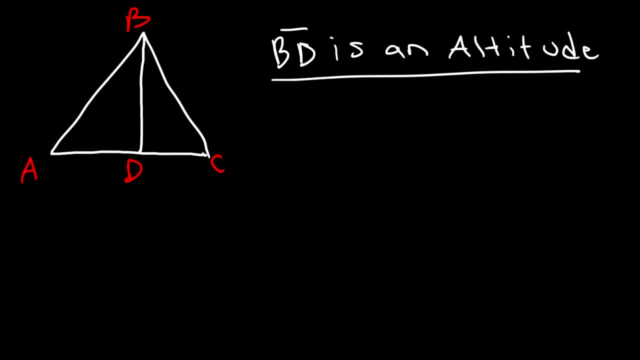 And what does it do? An altitude, like a median, is a line segment, But it differs from a median. It doesn't split the segment into two congruent parts. An altitude simply forms right angles, So an altitude is basically a line that's perpendicular to the other side. 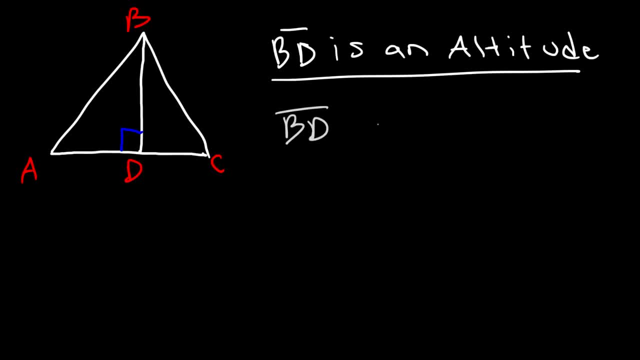 So BD is a line segment that's perpendicular to segment AC, And any time you have perpendicular lines it forms right angles. So angle ADB is congruent to angle CDB, Because they both equal 90 degrees, And so just make sure you understand that. 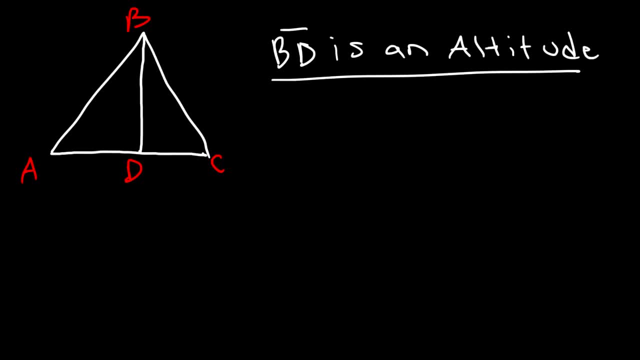 And what does it do? An altitude, like a median, is a line segment, But it differs from a median. It doesn't split the segment into two congruent parts. An altitude simply forms right angles, So an altitude is basically a line that's perpendicular to the other side. 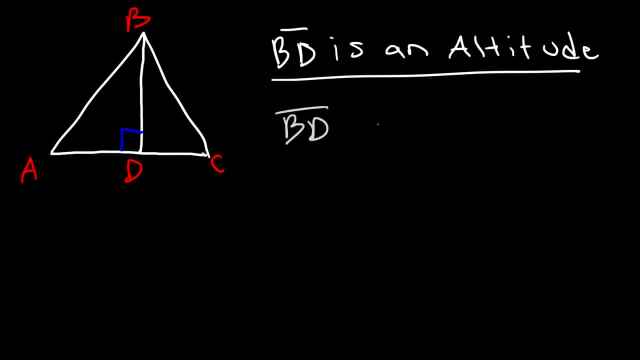 So BD is a line segment that's perpendicular to segment AC, And anytime you have perpendicular lines it forms right angles. So angle ADB is congruent to angle CDB, Because they both equal 90 degrees, And so just make sure you understand that. 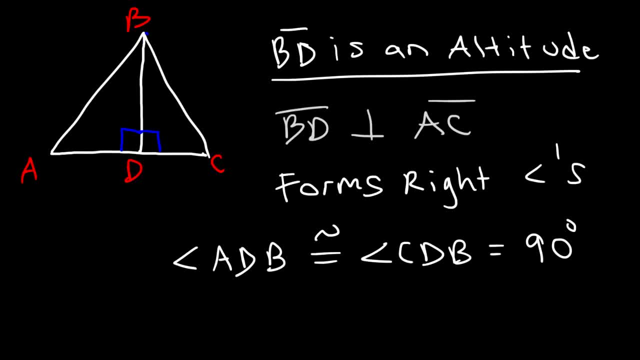 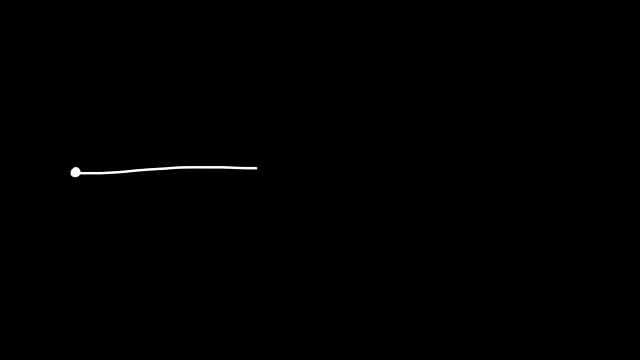 An altitude Simply connects- excuse me, connects- the vertex of one side of the triangle to the opposite segment, And it forms right angles. BD is perpendicular to AC. Now let's move on to perpendicular bisectors. So consider the segment AB. 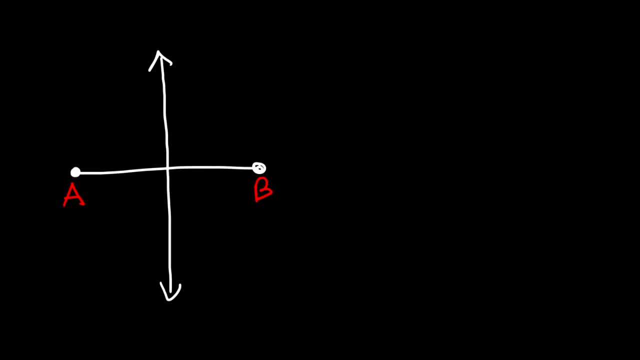 And we're going to draw a line that passes through it. Let's call this line L And let's say that line, Line L, is the perpendicular bisector of AB. So you can write it like this: Line L is the perpendicular bisector of segment AB. 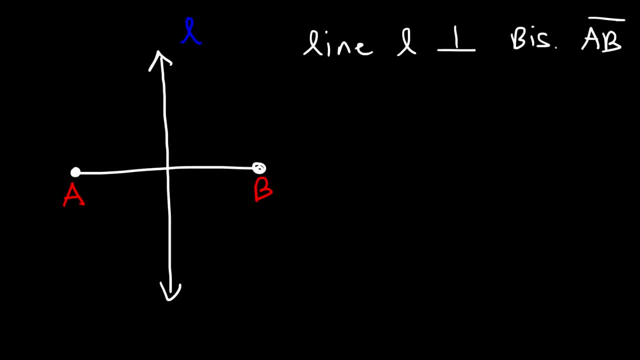 Now, perpendicular bisector is basically the hybrid of a median and an altitude combined. So like an altitude, it forms right angles And like a median, It splits the segment into two congruent parts. So let's call this point M. 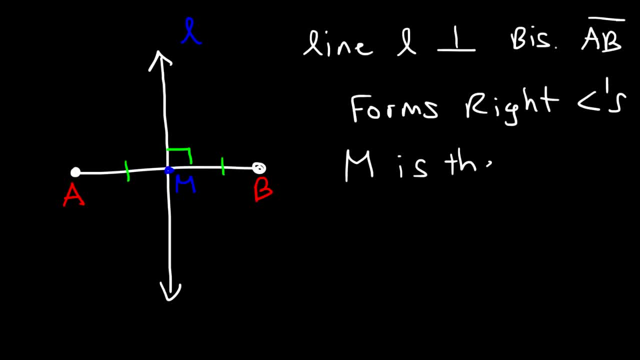 So therefore, M is the midpoint of segment AB And AM is congruent to BM. So the perpendicular bisector has features of an altitude and a median. But there are some other things you need to know about it. Let's say, if we put point P, 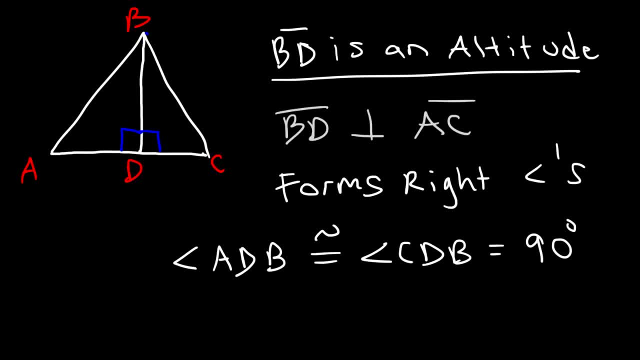 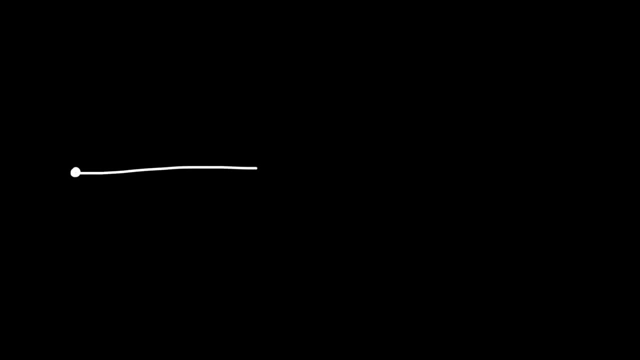 An altitude Simply connects- excuse me, connects- the vertex of one side of the triangle to the opposite segment, And it forms right angles. BD is perpendicular to AC. Now let's move on to perpendicular bisectors. So consider the segment AB. 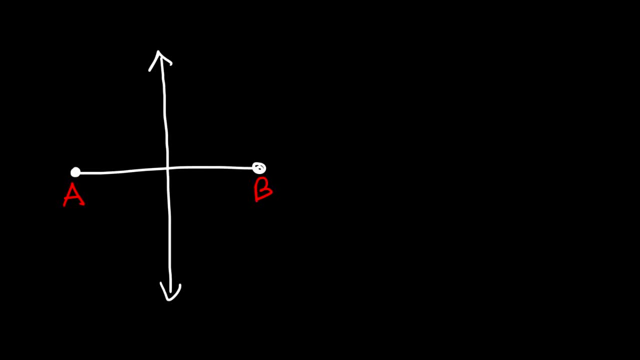 And we're going to draw a line that passes through it. Let's call this line L, And let's say that line L is a line segment. And let's say that line L is a line segment And let's say that line L is a line segment. 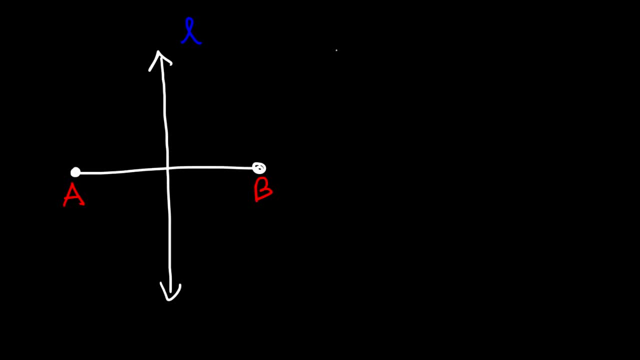 And let's say that line L is the perpendicular bisector of AB. So you can write it like this: Line L is the perpendicular bisector of segment AB. Now, perpendicular bisector is basically the hybrid of a median and an altitude combined. 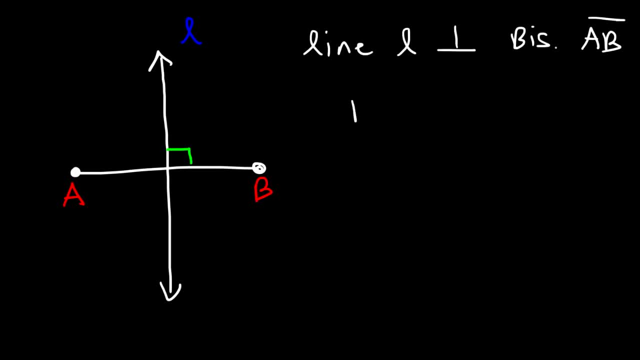 So, like an altitude, it forms right angles, And like a median, it forms right angles, And like a median, it forms right angles. It splits the segment into two congruent parts, So let's call this point M. So therefore, M is the midpoint of segment AB. 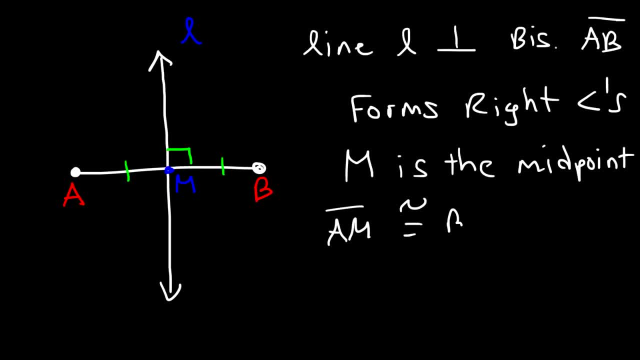 And AM is congruent to BM. So the perpendicular bisector has features of an altitude and a median. But there are some other things you need to know about it. Let's say, if we put point P and Q on the perpendicular bisector. 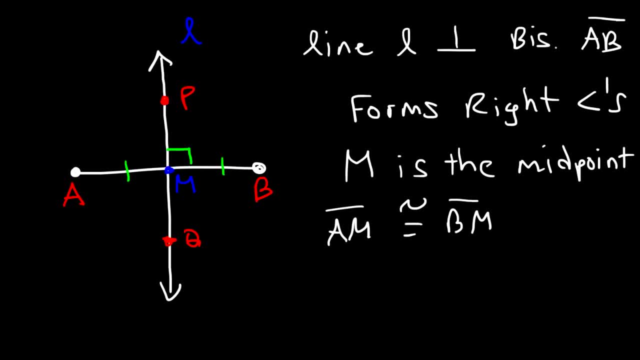 Any point on this line is going to be equidistant to the endpoints of the segment. So AP and BP are congruent, And also AQ is congruent to BQ. So notice that the perpendicular bisector forms congruent triangles. 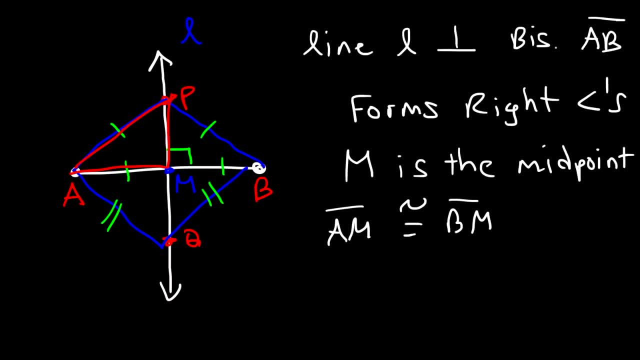 This triangle is congruent to that triangle. As you can see, this side is congruent to that side, This side is congruent to this side, And also the two triangles share a common side, Which is equivalent based on the reflexive property. 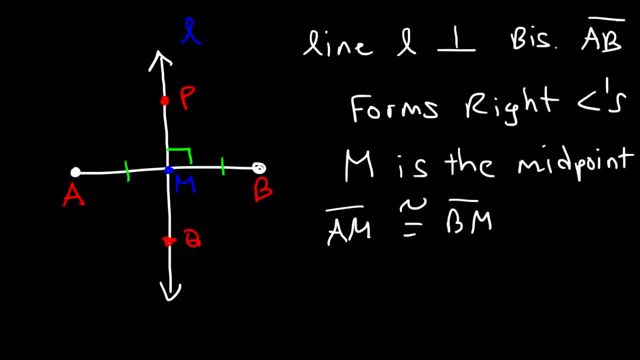 And Q on the perpendicular bisector. Any point on this line is going to be equidistant to the endpoints of the segment. So AP and BP are congruent, And also AQ is congruent to BQ. So notice that the perpendicular bisector forms congruent triangles. 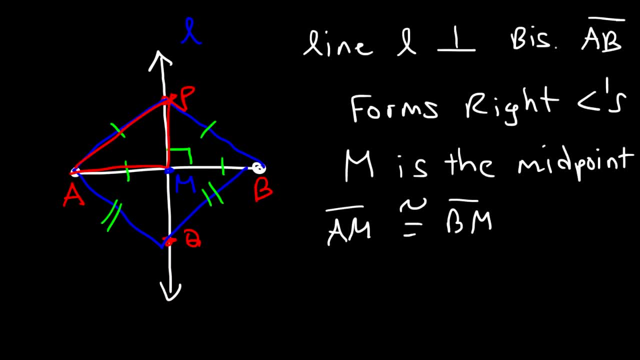 So this triangle is congruent to that triangle. As you can see, this side is congruent to that side, This side is congruent to this side, And also the two triangles share a common side, Which is equivalent, based on the reflexive property. 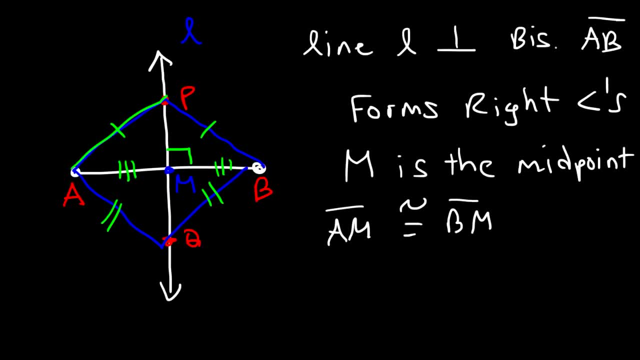 So by the SSS postulate you can prove that these two triangles are congruent. Now if you can show that these two points are equidistant to the endpoints of the segment, Then these two points, they form the perpendicular bisector of segment AB. 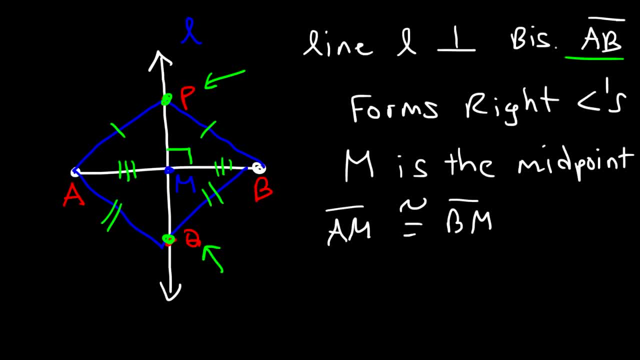 Because sometimes you have to prove that line is the perpendicular bisector And to do that you have to show that these two points are equidistant to A and B. So therefore, line PQ is congruent to the segment AB. So this is the perpendicular bisector of segment AB. 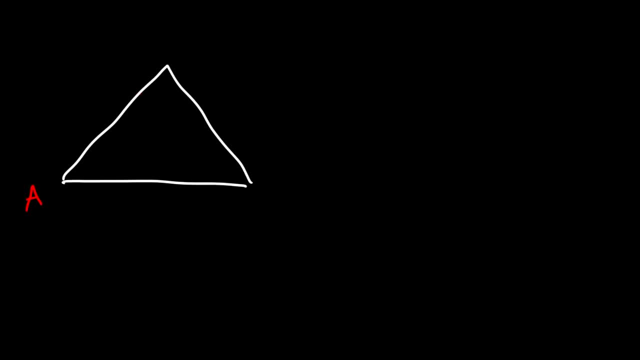 Now, the next thing that we need to talk about is an angle bisector. So let's say that BD is an angle bisector of ABC. What conclusions can we draw? Now? an angle bisector is a power. Now, an angle bisector is a power. 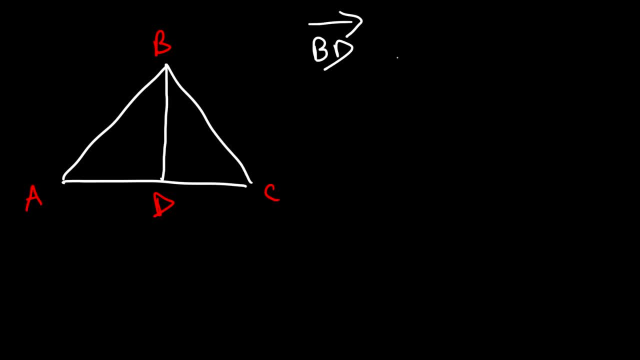 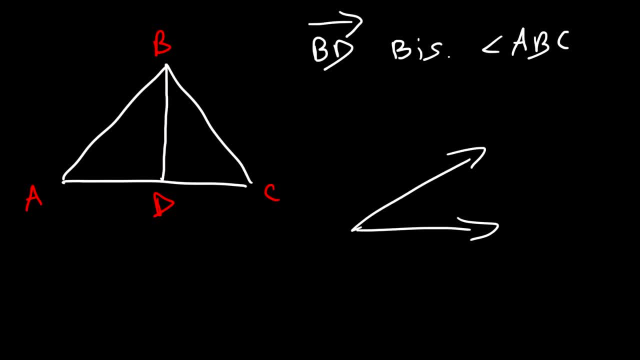 an angle, you need to connect two rays to it, So two rays are necessary to form an angle. This is the vertex of the angle, also known as the common endpoint. So let's say this is ABC, So that's angle ABC, And then another ray is used to divide ABC into two congruent parts. 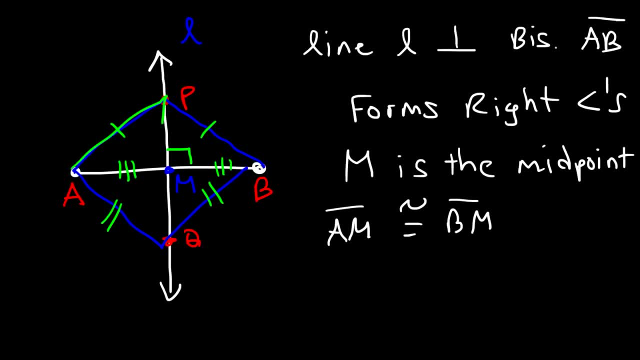 So by the SSS postulate you can prove that these two triangles are congruent. Now if you can show that these two points are equidistant to the endpoints of the segment, then these two points, they form the perpendicular bisector of segment AB. 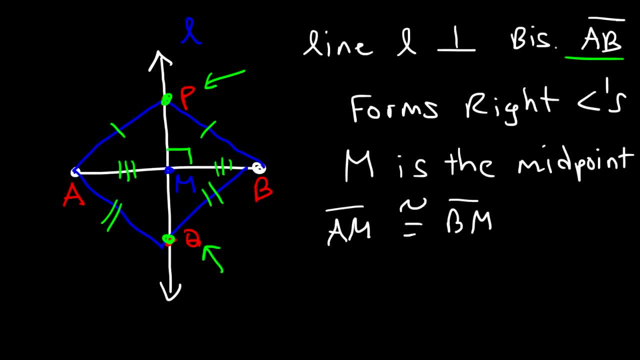 Because sometimes you have to prove that line is the perpendicular bisector, And to do that you have to show that these two points are equidistant to A and B. Therefore, line PQ is the perpendicular bisector of segment AB. Now the next thing that we need to talk about is: 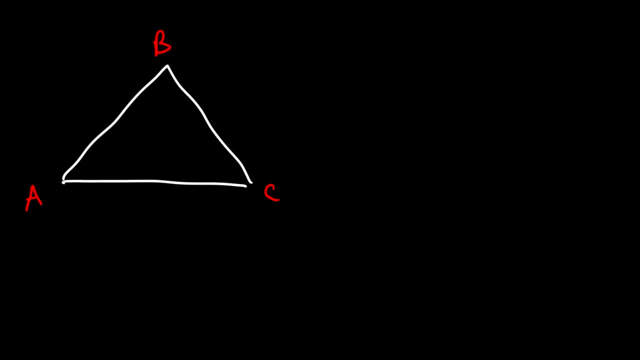 an angle bisector. So let's say that BD is an angle bisector of ABC. What conclusions can we draw Now? an angle bisector is a ray, So angle- I mean ray- BD bisects angle ABC. If you think about it, whenever you need to form an angle, 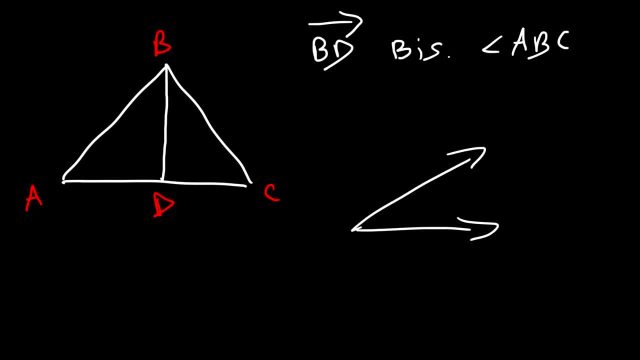 you need to connect two rays to it, So two rays are necessary to form an angle. This is the vertex of the angle, also known as the common endpoint. So let's say: this is A, This is ABC, So that's angle ABC. 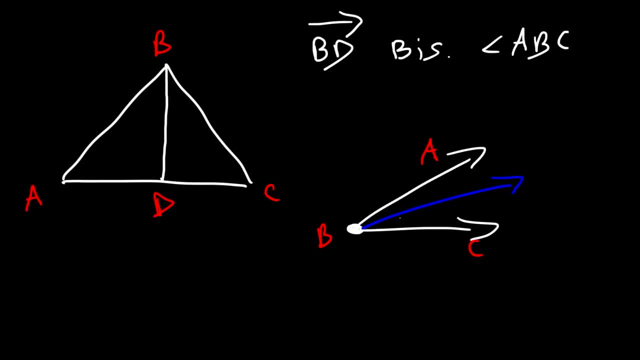 And then another ray is used to divide ABC into two congruent parts. Let's call this BD, So ray BD bisects angle ABC. So these two angles are congruent, So we can make the conclusion that angle ABD. 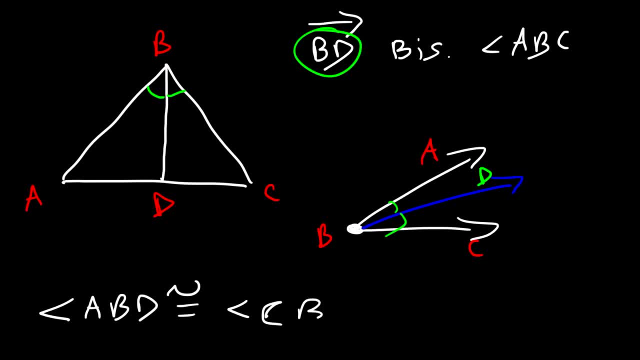 is congruent to angle CBD, And so that's the definition of an angle bisector. It simply bisects the angle into two congruent parts. So you draw it starting from the vertex of an angle, I mean of a triangle. 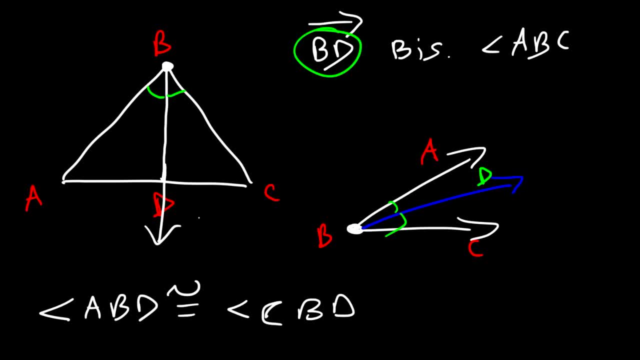 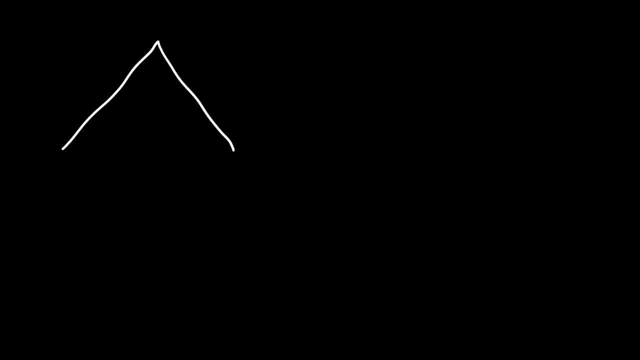 And then it points to the opposite side. But angle bisectors, by definition, are rays. So I'm going to give you a mini quiz. I'm going to draw four triangles And the line in the middle I want you to determine. 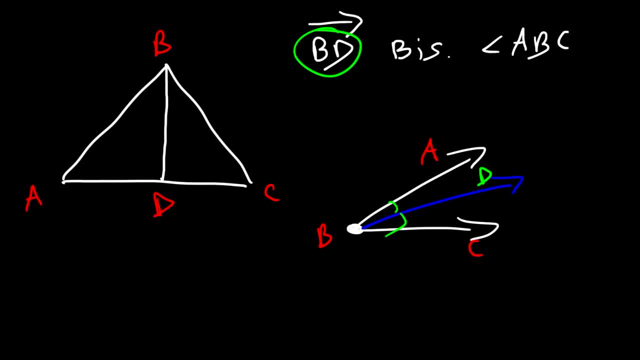 Let's call this BD, So ray, BD bisects angle ABC. So these two angles are congruent. So we can make the conclusion that angle ABD is congruent to angle CBD, And so that's the definition of an angle bisector. 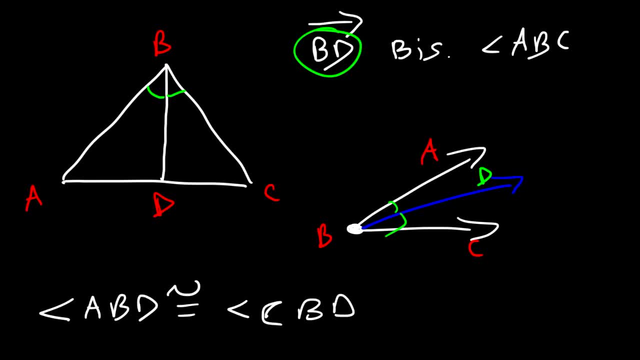 It simply bisects the angle into two congruent parts. So you draw it starting from the vertex of an angle- I mean of a triangle- and then it points to the opposite side. But angle bisectors by definition are rays. 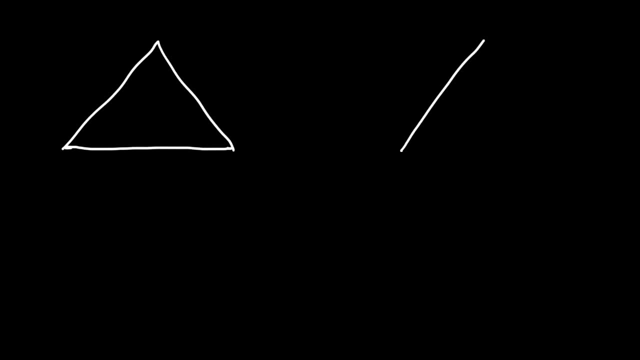 So I'm going to give you a mini quiz. I'm going to draw four triangles And the line in the middle I want you to determine if it's altitude, A median, a perpendicular bisector or an angle bisector. So let's call this ABCD. 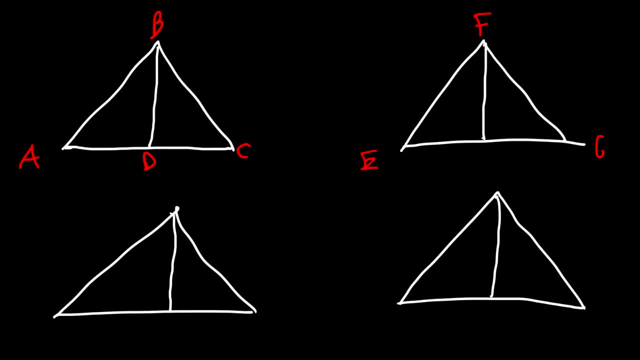 And let's say this is EFGH, Let's say this is JKLM And QKLM And this is RST. So let's say this is a right angle. Let's say this is a right angle and this side is congruent to that side. 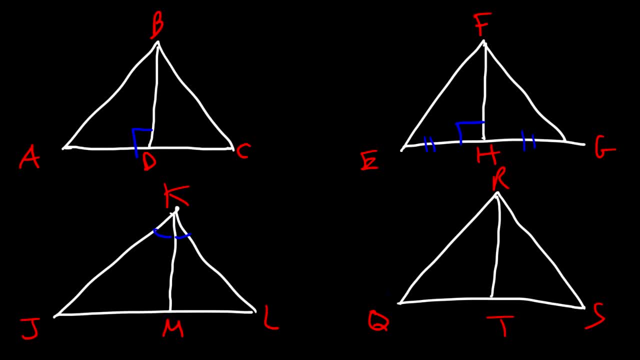 And let's say these angles are congruent And QT is equal to TS, So which one is a median? Is it BD, FH, KM or RT? So feel free to pause the video and identify the median, The median. all it does is it splits a segment into two congruent segments. 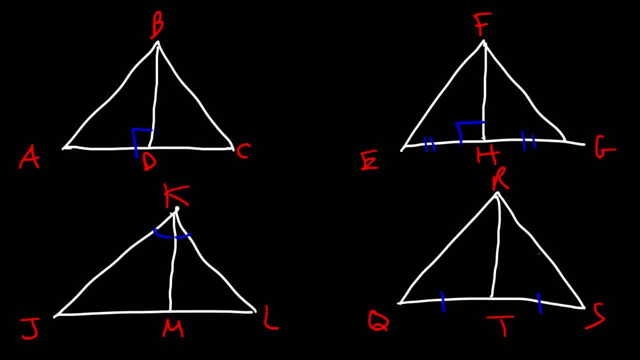 So that represents the fourth picture. So therefore, RT is a median. Now which one is the altitude An altitude? all it does is it forms right angles. So BD is an altitude. Now which one is the angle bisector? 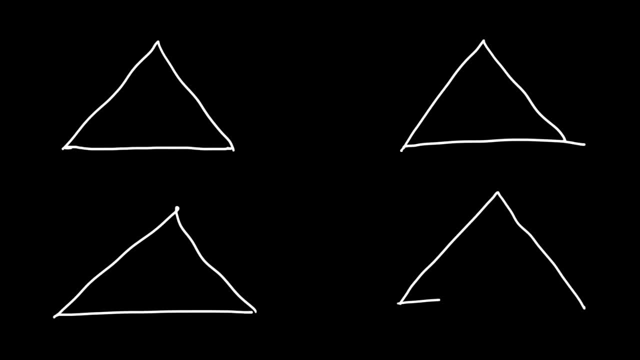 if it's an altitude, a median, a perpendicular bisector or an angle bisector. So let's call this ABCD And let's say this is EFGH. Let's say this is JKL, Okay, So let's say this is LLM and QRST. 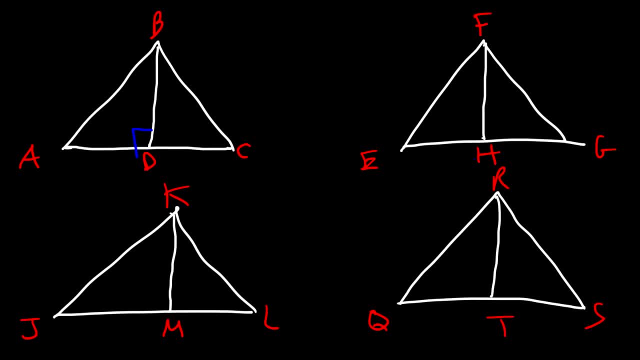 So let's say: this is a right angle. Let's say this is a right angle and this side is congruent to that side. And let's say: these angles are congruent And QT is equal to TS, So which one is a median? 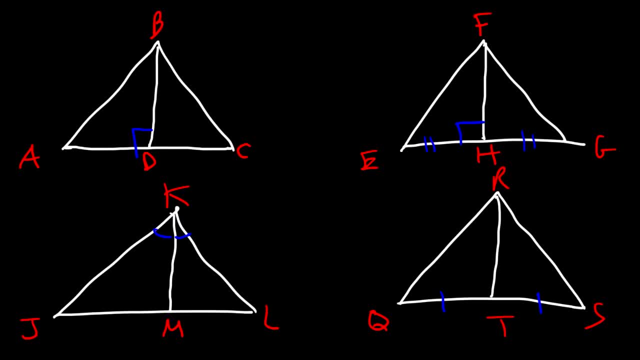 Is it BD, FH, KM or RT? So feel free to pause the video and identify the median. The median. all it does is it splits a segment into two congruent segments. So that represents the fourth picture. So therefore, RT is a median. 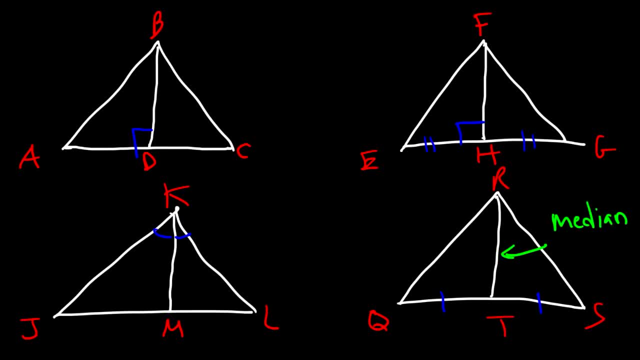 Now which one is the altitude? An altitude. all it does is it forms right angles. So BD is an altitude. Now, which one is the angle bisector? Now, this one is straightforward, because it bisects angles, So KM is the angle bisector. 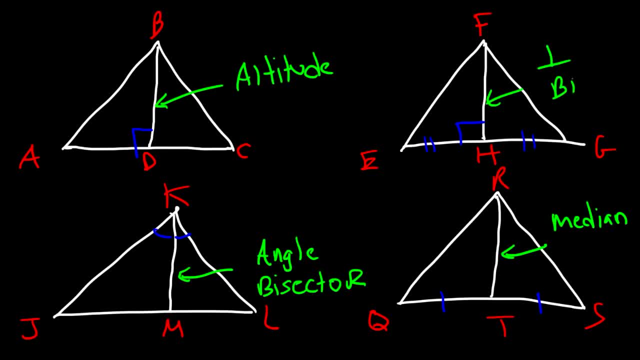 And the last one is the perpendicular bisector. So altitudes and medians are line segments. An angle bisector is a ray, It starts from K and points towards M, And a perpendicular bisector is a line. So that is it for this video. 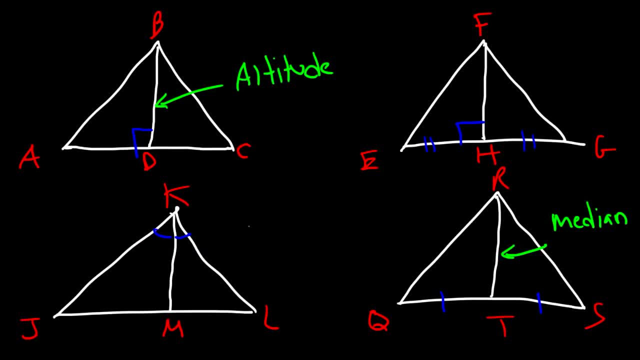 Now, this one is straightforward because it bisects angles. So KM is the angle bisector And the last one is the perpendicular bisector. So altitudes and medians are line segments. An angle bisector is a right angle bisector. 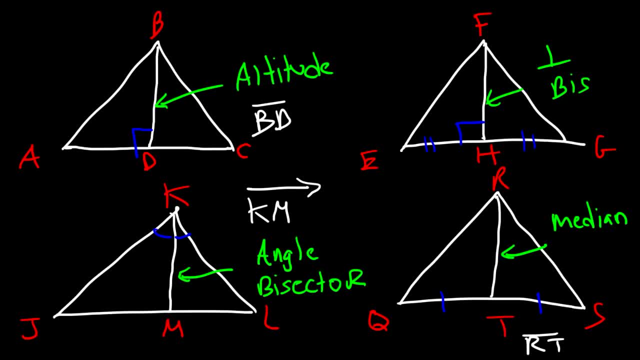 An angle bisector is a right angle bisector. An angle bisector is a right angle bisector And a perpendicular bisector is a right angle bisector. It starts from K and points towards M, And a perpendicular bisector is a line. 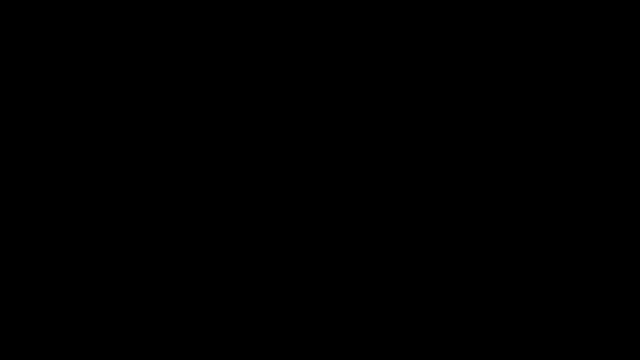 So that is it for this video. If you want to find more of my geometry video tutorials, just visit my channel and you can access the playlists, which I try to organize the videos in order so you can follow it based on the course of your class. 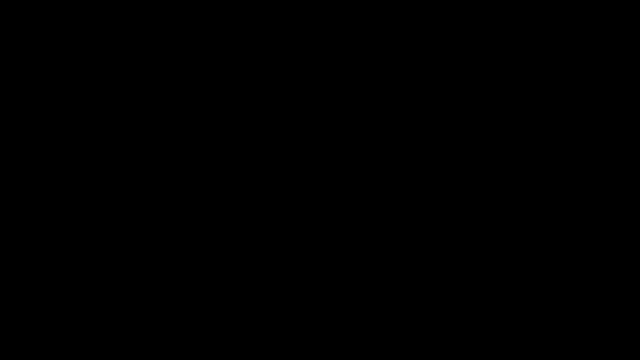 Subtitles by the Amaraorg community. So if you liked this video, let me know, feel free to comment, and thanks for watching. 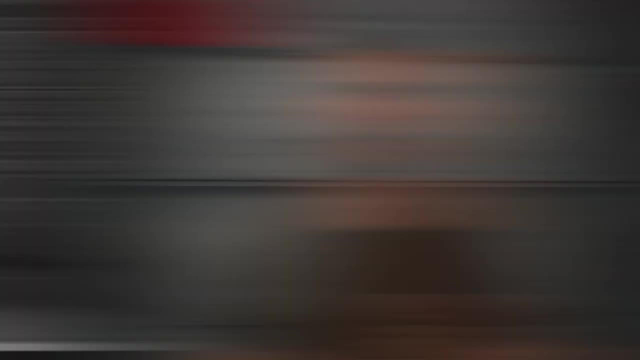 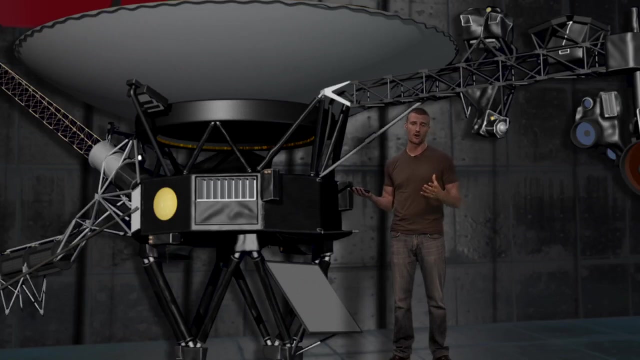 Hey everybody, Technology is always getting smaller. A computer used to take up an entire room, but now it fits in the palm of your hand. Well, spacecraft aren't all that different. They're traditionally very large and difficult to build, but we're working on ways to miniaturize them. 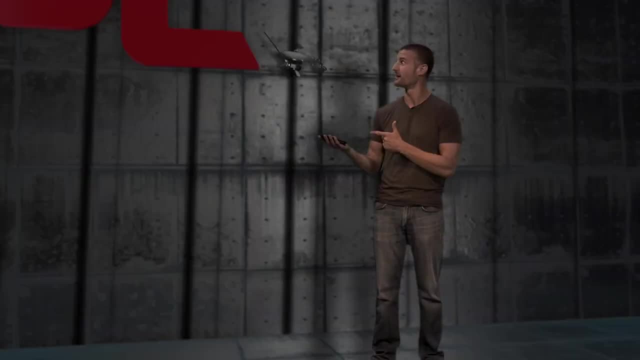 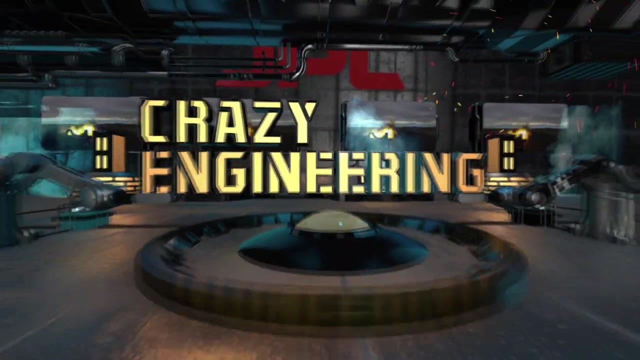 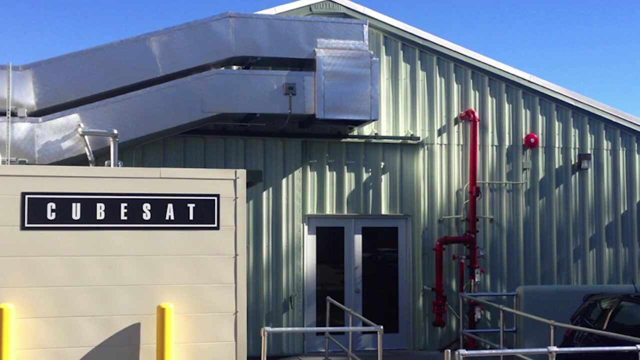 We're going to talk all about that on this episode of Crazy Engineering. Hey everybody, We're here with Andy Klesch in one of JPL's smaller clean rooms. We're building CubeSats in here. Andy, what exactly is a CubeSat? 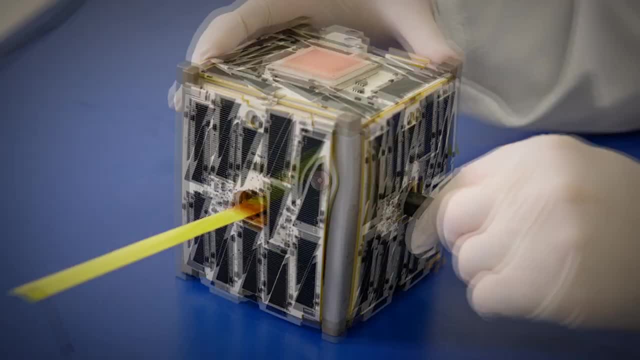 A CubeSat is really just a standard for a small spacecraft, And we're talking a very small spacecraft: 10 by 10 by 10 centimeters at the smallest on here, And yet they go up to about 30 by 20 by 10 centimeters. 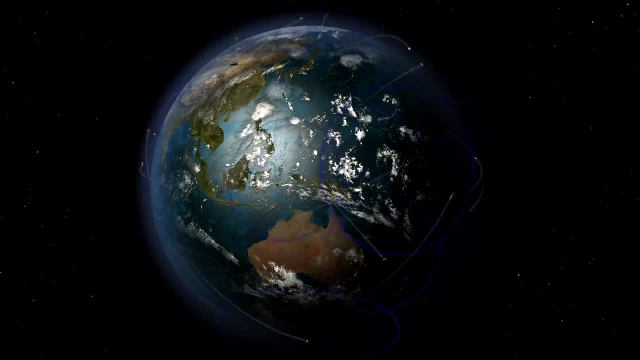 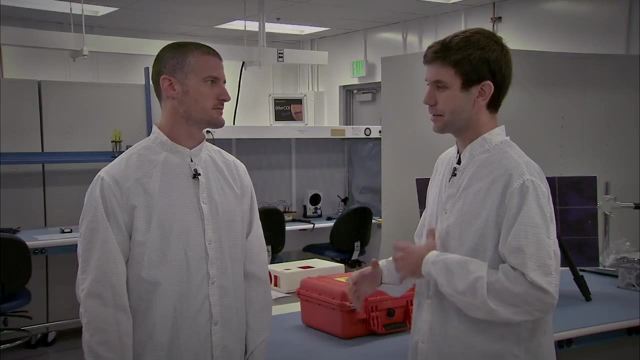 And we've launched hundreds into low Earth orbit for the last 10, 15 years. So this really is in a big contrast to how we normally operate at JPL with our larger clean rooms and our larger spacecraft. It is We're trying things a little bit different over here. 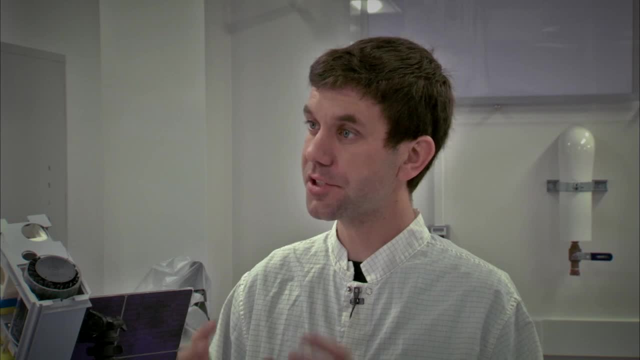 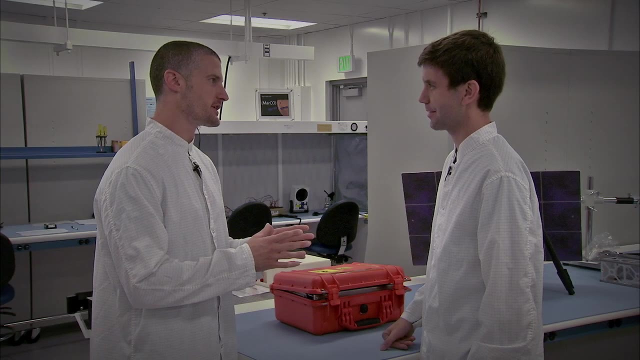 Absolutely not. Voyager has so many different capabilities And these CubeSats are very, very limited, but they're very focused on what they do, So they can do one thing and do it very, very well. You're the chief engineer of one of these.